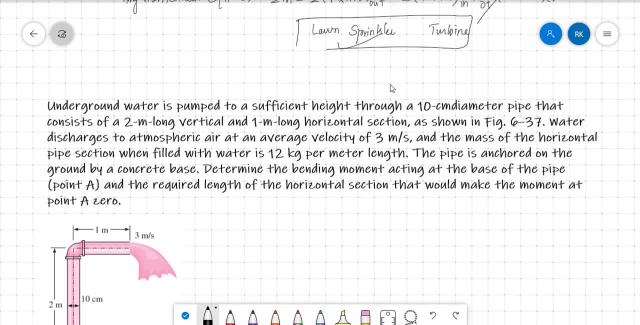 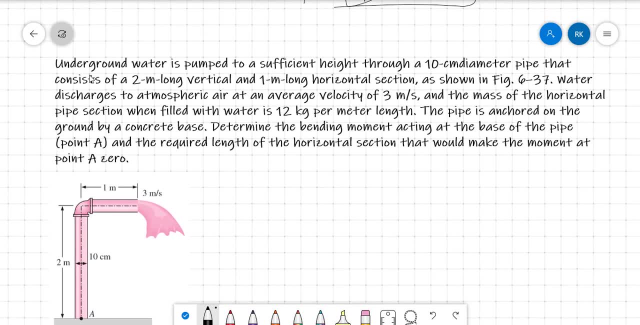 EAC. so, in order to understand that, let us see this example. first let us see this example and then we will move to launch sprinkler. the question is: underground water is pumped to a sufficient height through a 10 cm diameter pipe that consists of a 2 m long vertical and 1 m long horizontal section, as shown in the figure. 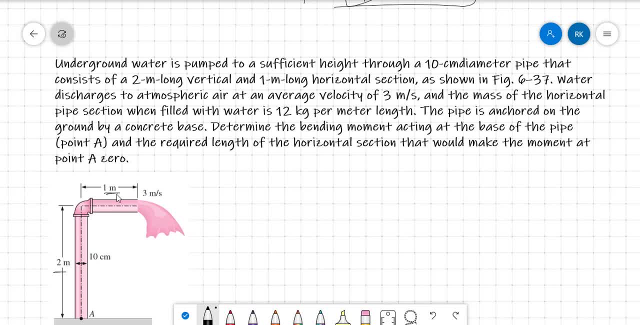 so this is 2 m long and this is 1 m. horizontal water discharges to atmosphere air at an average velocity of 3 m per second and the mass of the horizontal pipe section when filled with water is 12 kg per meter length. the pipe is anchored on the ground by a concrete base. so here there. 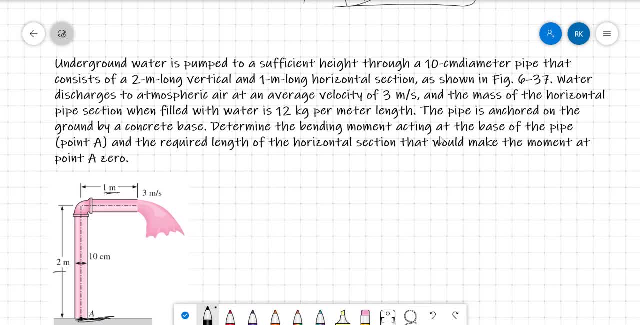 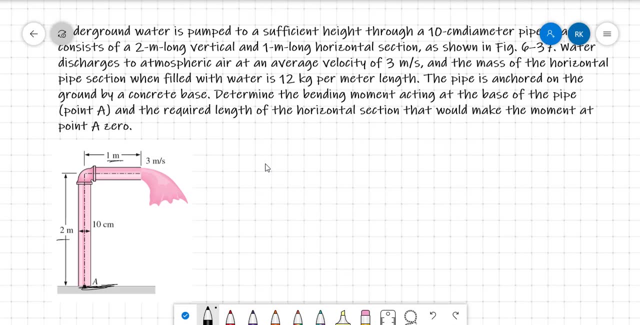 is attachment: determine the bending moment acting at the base of the pipe, point A- and required length of the horizontal section. that would make the moment at point, moment at point A, zero. so the question asked here is: determine the bending moment acting on the base. So this is: what is the bending moment that is acting? so what is the bending moment in? 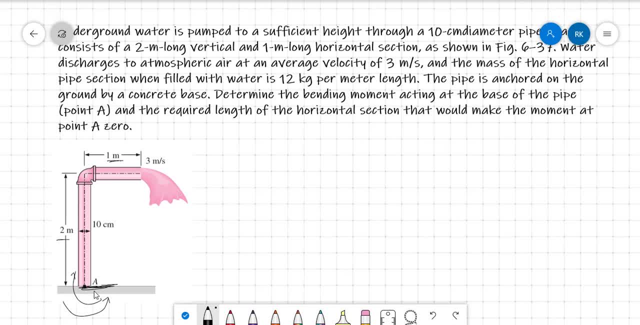 this direction, or clockwise or anticlockwise, and also we need to find the magnitude of the moment and we need to find the required length of horizontal section. so how much this length of horizontal section should be maintained, so that here the resistance moment will be zero? 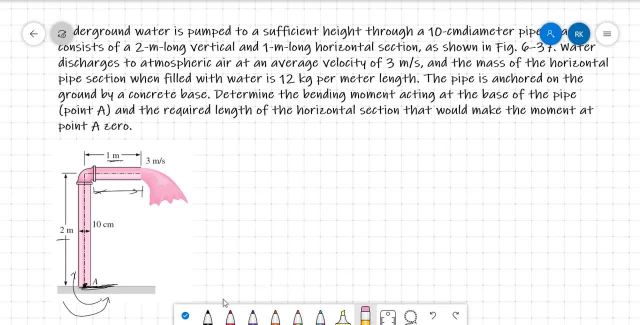 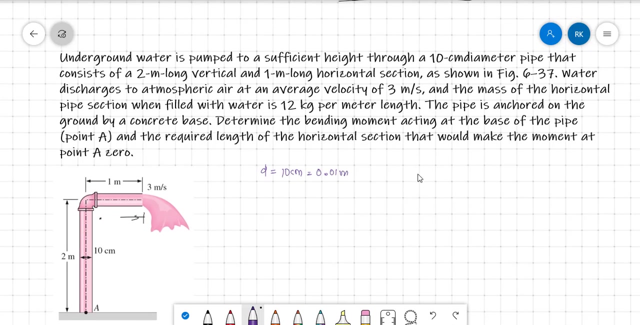 So let us see now. So So Solve this. let me write the given data first. So underground water response to the diameter of the pipe is: diameter is equal to 10 centimeter, which is equal to 0.01 meter, and that consists of 2 meter long vertical and 1 meter long. 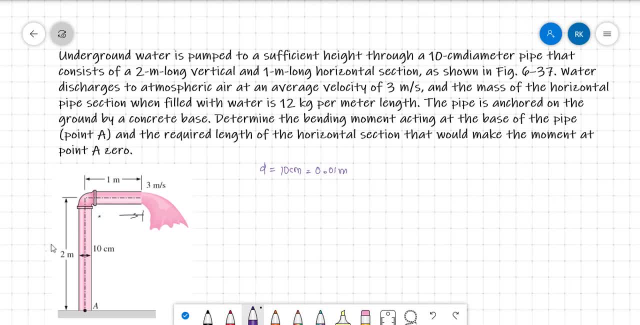 horizontal section. Let me say this is R1 and this is R2.. So R1- I am considering up to this point- the weight will be the weight of this horizontal section, with the water will be at this point and this is R1.. So R1 is equal to 0.5 meter. 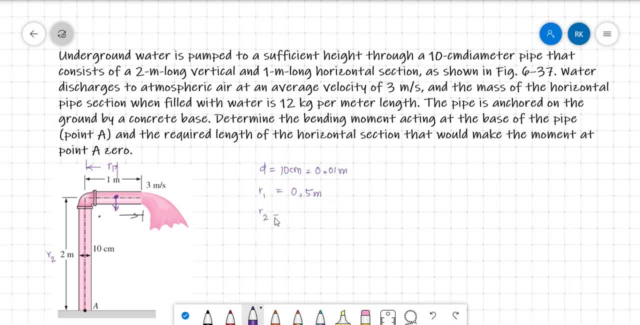 And R2 will be 2 meter. So water discharges to atmospheric weight at the velocity the velocity is. velocity is equal to 3 meter per second and the mass of horizontal 12 kg per meter length. W is equal to 12 kg per meter. 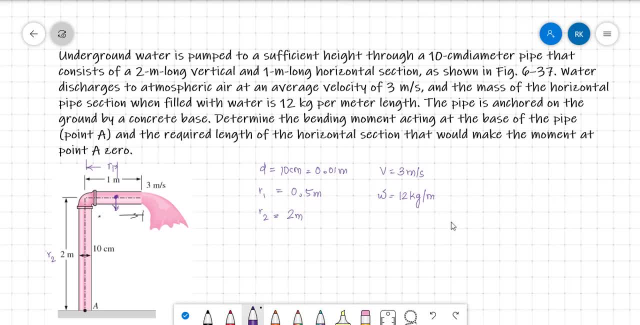 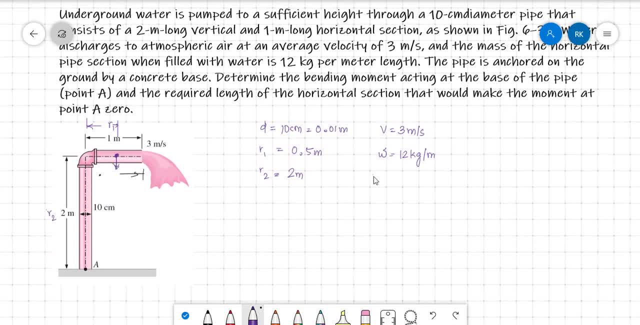 So these are- this is the given data, and consider that row of water is 1000 kg per meter cube. 1000 kg per meter cube, So we need to apply angular momentum equation. angular momentum equation. So considering this as a steady flow one. 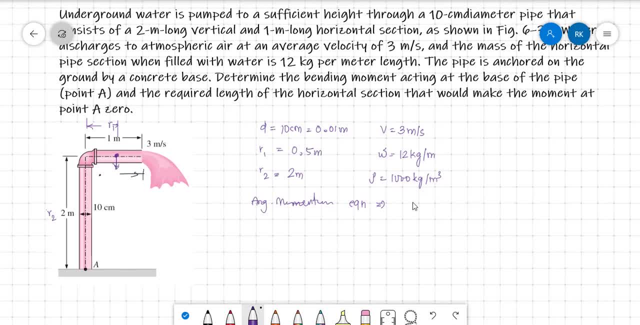 If nothing is given, consider it as a steady flow. If nothing is given, consider it as a steady flow. So, summation of moments. This is solid moments, Solid moment, Which means a resisting moment that is due to the solids, which is equal to summation. 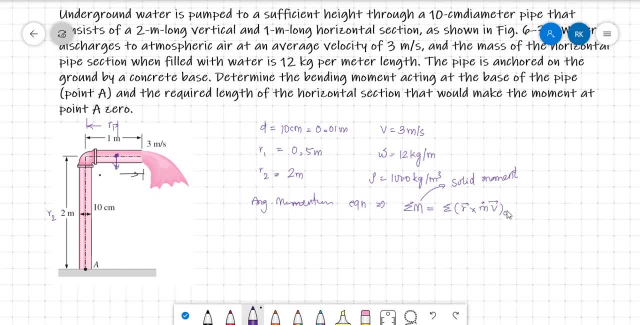 of Outside movements Today. Outside movement: fluid inside that is flowing inside moment here. if we see, considering moment about this point, the flow, considering this as the control volume. so this has a control volume. the flow inside is in this way so there will be R bar is 0, so 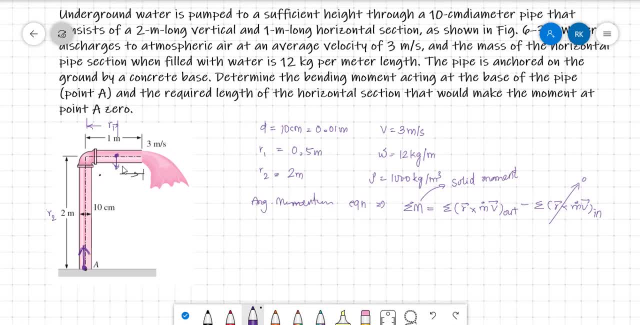 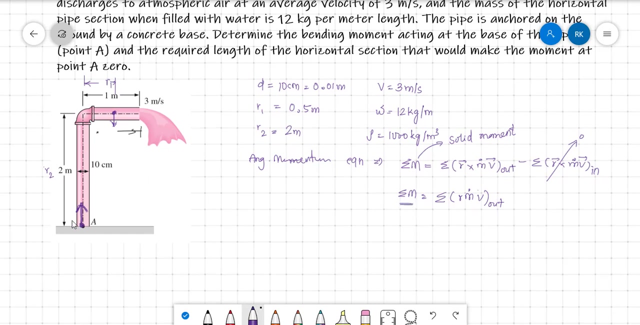 inside, inside momentum will be 0 and outside momentum- here we are not considering the vector case. so Sigma M is equal to summation of R M dot V outside. so here summation of moments, let me say I am considering this resisting moment is in this way and I am saying that: 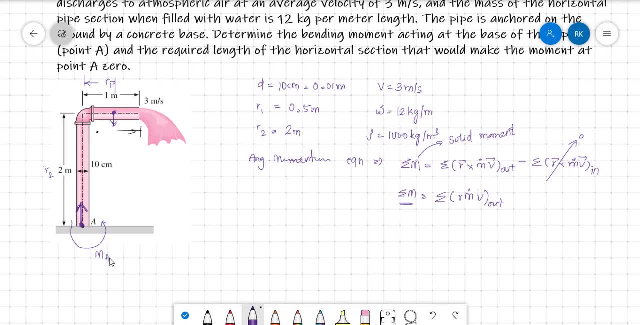 MA. so what are the solid moments that are acting? so, MA, the resisting moment is acting. I am considering the clock anticlockwise as negative, so minus MA. and the another solid moment is due to this weight. so that is this one, due to this, about this point a: it is clockwise, so positive plus weight of the pipe with. 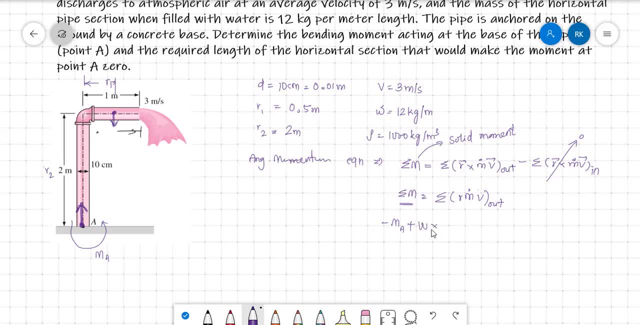 the water into how much is the perpendicular distance? that is, R 1 is equal to summation of this that water flowing outside. so from where water is flowing outside through this section, so that one flow, so M dot into velocity is 3 meter per second, into R. So this R2 is the perpendicular distance of this velocity. So 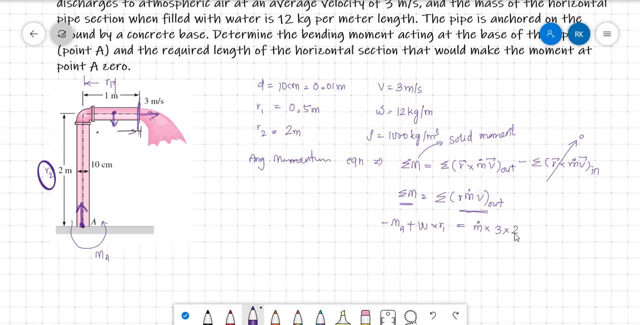 that is 2 meter. So what should be the sign? So this is going outside and about this point, that is clockwise, So that will be positive. Finally, MA moment, the resisting moment at A is equal to 6 into M dot. What is M dot? M dot is equal to Rho A V, So density is 1000. 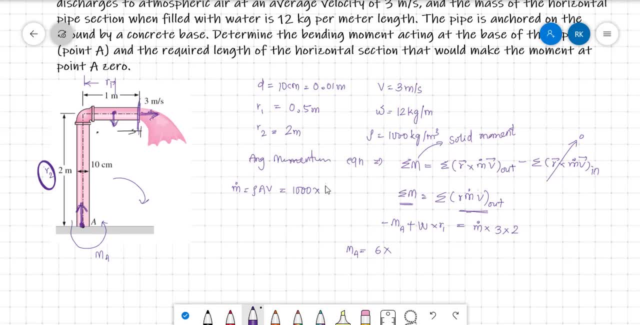 kg per meter cube and area of cross section pi by 4 into d square, into velocity, So that is 3 meter per second. So M dot will be 23.56 kg per second. So M dot is equal to 23.56.. 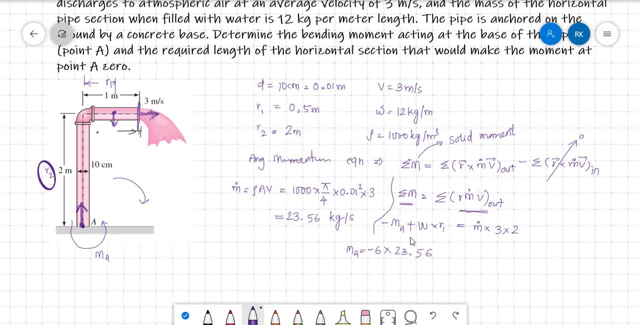 So this is MA, So this will be minus plus W. What is W? This is 1 meter length, So W of horizontal 1.. That is equal to 12 kg per meter. into how much length it is 1 meter length. So 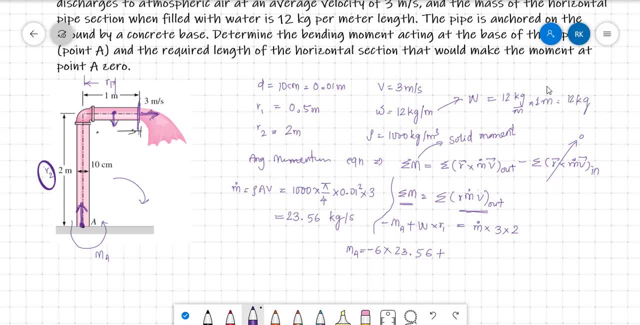 12 kg into 9.81 gives us weight. So 12 into 9.81 is 118 Newton. So 118 into. So the weight will be acting At the center of gravity, So that will be equal to R1.. That is 0.5 meter 0.5.. So the MA will be. 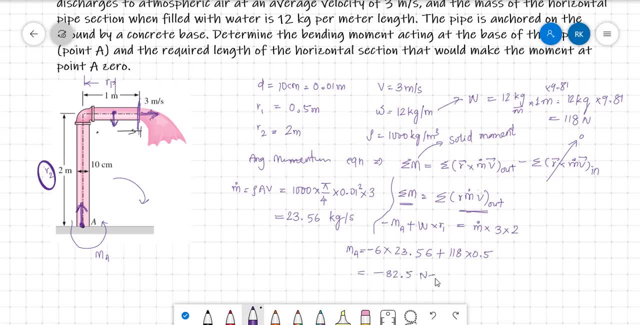 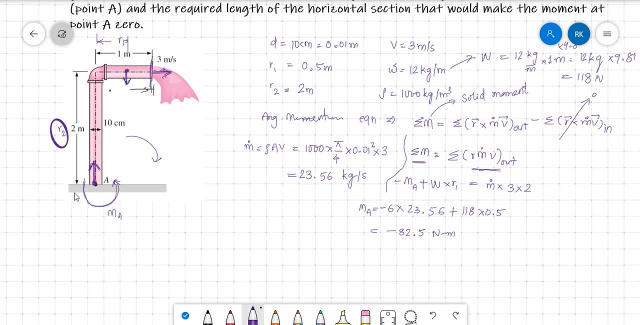 minus 82.5 Newton meter. So what it is indicating, Our consider direction, is wrong and the actual direction should be in this way. The actual direction of movement is this one, not this. So the moment with MA is equal to 82.5 Newton meter, counterclockwise. 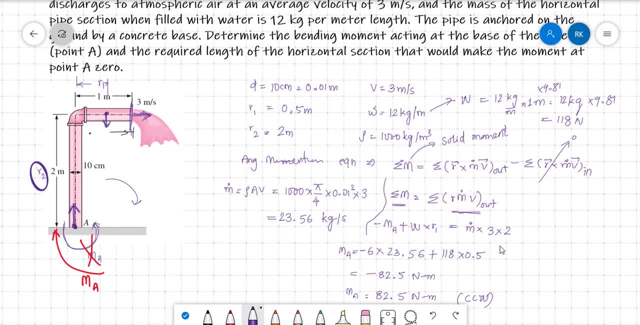 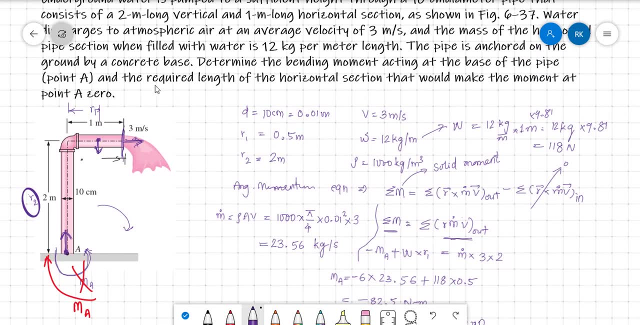 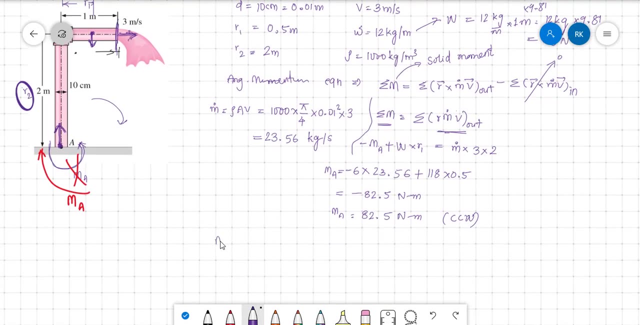 so this is the moment and it's a rotation counterclockwise. and the second question is the required length of the horizontal section. that would make the moment at point a 0. so in order to make moment at a, the resisting moment should be 0. so how much length, how much horizontal length should be kept? so 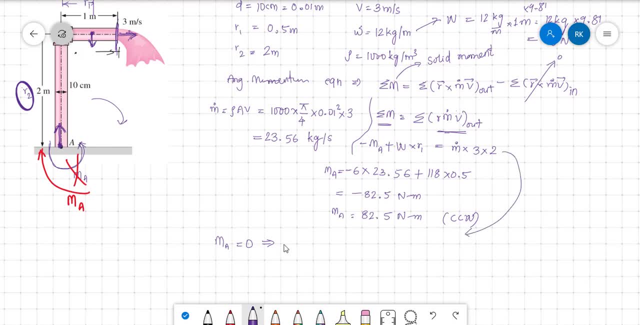 substituting this, so MA is equal to 0, 0 plus W. W is W into L. this is weight per unit length and how much length should be maintained. is L, W into L? what is R 1? R 1 is length of the pipe divided by 2. center of gravity will be length of the. 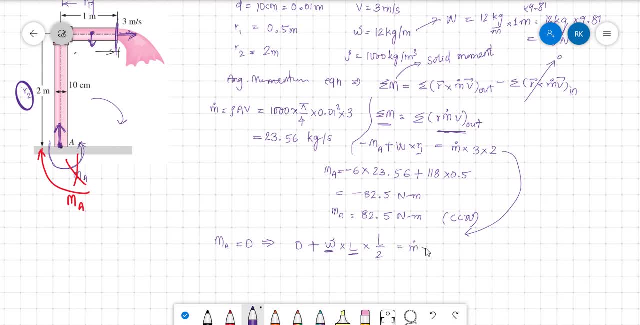 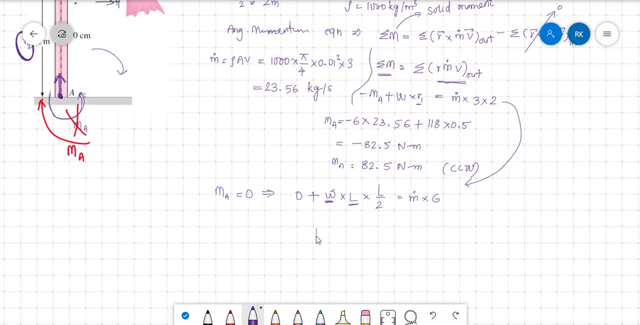 pipe, divided by 2, that is equal to M dot into 6. so W, what is W, 12 kg per meter into nine point eight. one. that is the unit weight per unit length into L. square by 2 is equal to M dot into six M dot. M dot is twenty three point five, six into six. 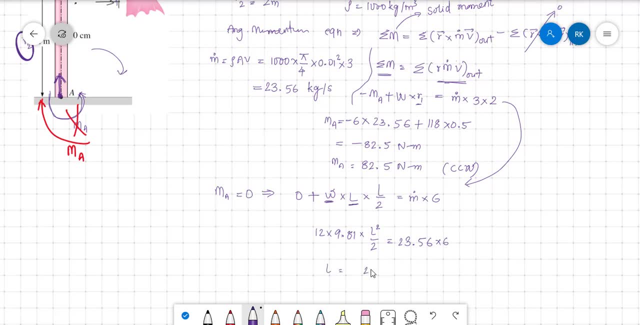 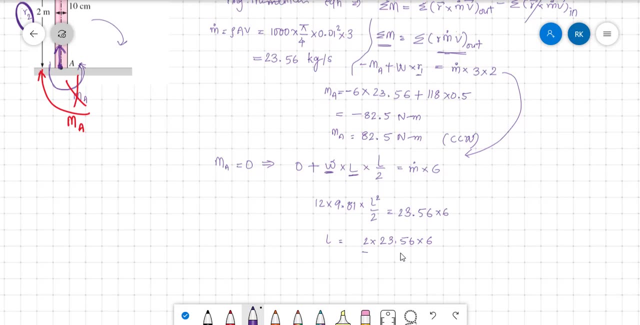 so L is equal to two into twenty, three point five, six into six, divided by twelve into nine, point eight, one under root of this one. so by solving this we will be getting two point four meter. so if we keep this horizontal pipeline, 2.4 meter. 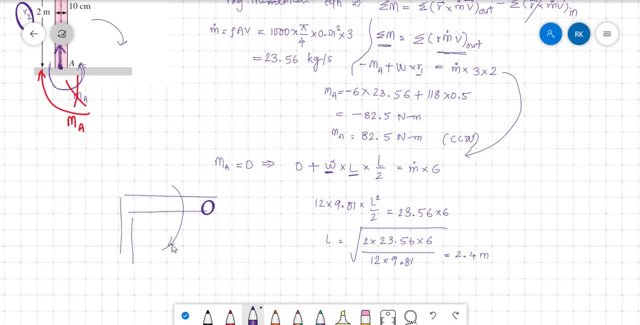 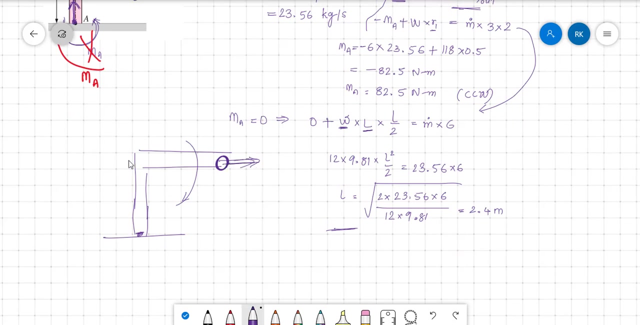 so this will be M acting in this way about this point. so this is clockwise moment and due to this and due to this, both will be balanced. due to this one, there is the reverse moment that will be created. so this, both should this, both are balanced and there. 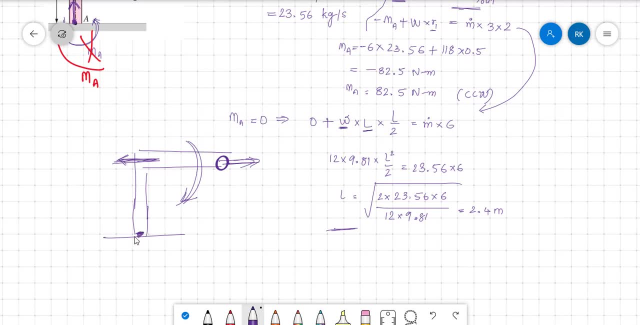 will be no moment that will be acting here. if you observe, due to this out outside flow, there is a reverse impact that is created if you look in rockets. so the flow, the fluid flow, is downside, but rocket is moving upside in this way, in the same sense. 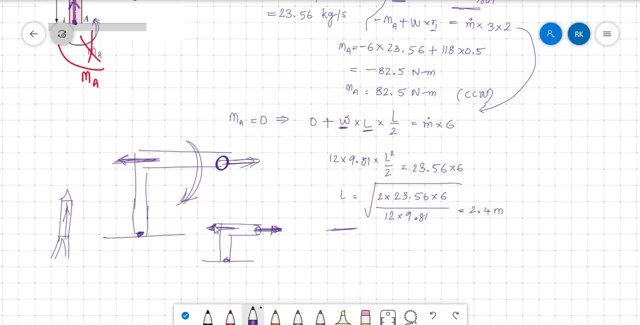 if the velocity is in this direction, there will be a force that will be acting in this direction and, due to this, the moment will be in this, in this way, and there to resist that, the moment will be. the moment here downward will be this way, but here, in this case, there is another moment in this way, so this one: 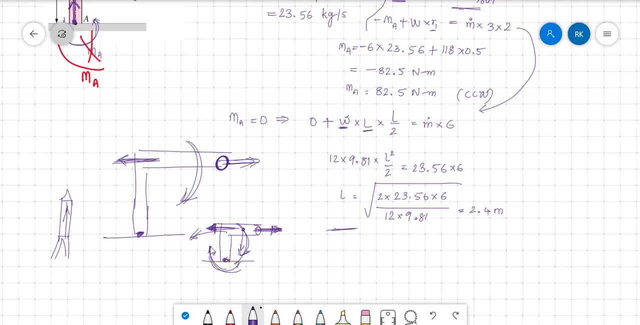 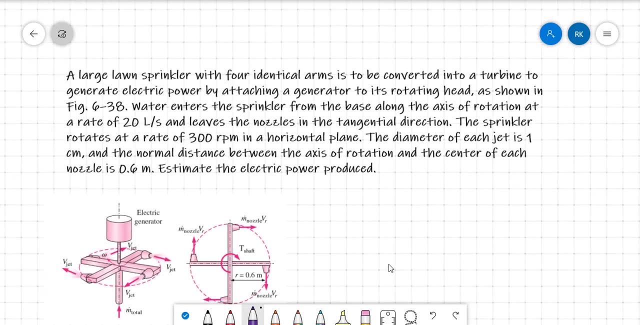 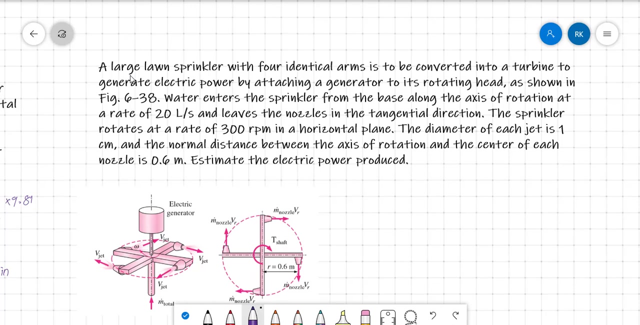 is very large, so that the moment change in its direction this way, so we will see no lawn sprinkler. with an example, a large lawn sprinkler with four identical arms is to be converted into a turbine to generate electric power by attaching a generator to its rotating head, as shown in the 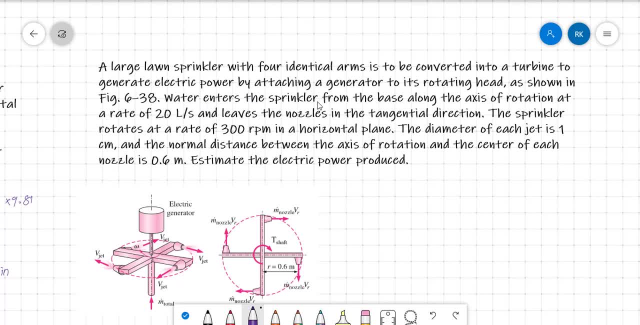 figure water enters the sprinkler from the base along the axis of rotation at 20 liter per second and leaves the nozzles in the tangential direction. water enters the sprinkler from the base along the axis of rotation at 20 liter per second and leaves the nozzles in the tangential direction. 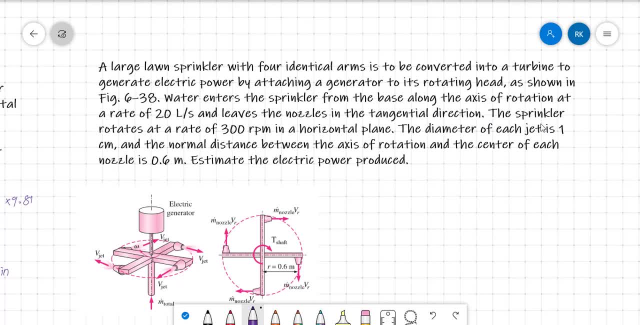 the sprinkler rotates at a rate of 300 rpm in a horizontal plane. the diameter of each jet is 1 centimeter and the normal distance between the axis of rotation and center of each nozzle is 6 meter. sorry, 0.6 meter. estimate the: 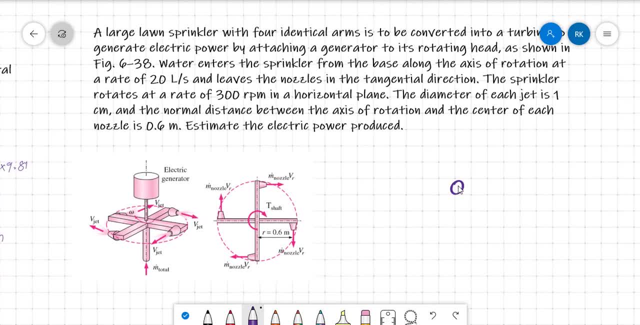 electric power produced. so what is lawn sprinkler? so if, if any liquid is supplied through this, it is distributed to this one and this one. due to this, because of this, it is distributed to this one and this one. due to this, if any liquid is supplied through this, it is distributed to this one and this one. due to this. 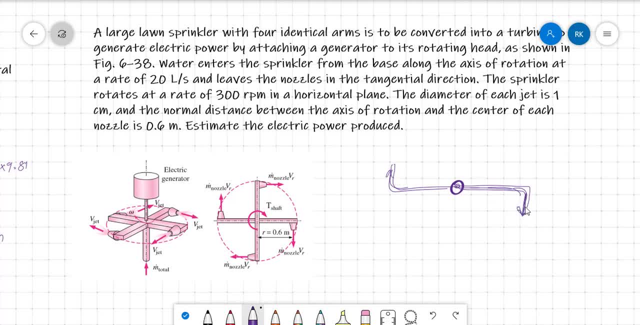 if this fluid is flowing outside in this way, as I said, there is an opposite impact that will be created and this will be rotating in this direction. due to this, this will be rotating in this direction, so there is a counterclockwise rotation that will be created. so, due to this, 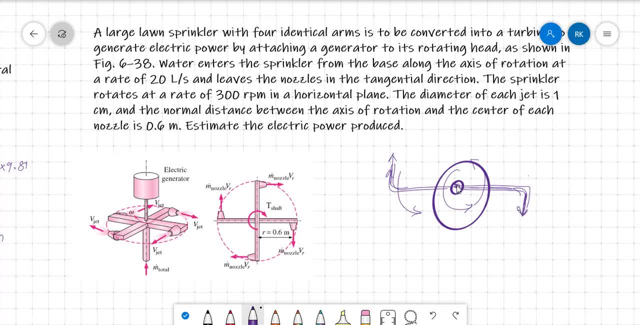 creation. if we connect this point to generator, there will be electricity produced. so in order to produce electricity, there will be, there should be a torque, that should be created. so we need to find that torque. so here water is supplied, from here this point, and from four nozzles the water comes out. 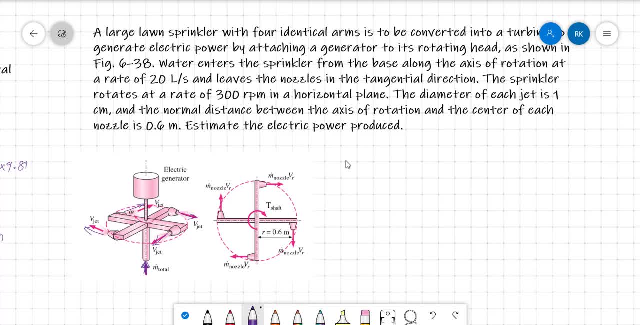 with a velocity. so first let me write the given data. water in this fountain is GW to 20hana per second, so discharge is equal to 20 liter per second and leaves theijels in the tangential direction, so in unusual direction, that is, living. the sprinkler rotates at a speed, at a rate of 300 rpm. 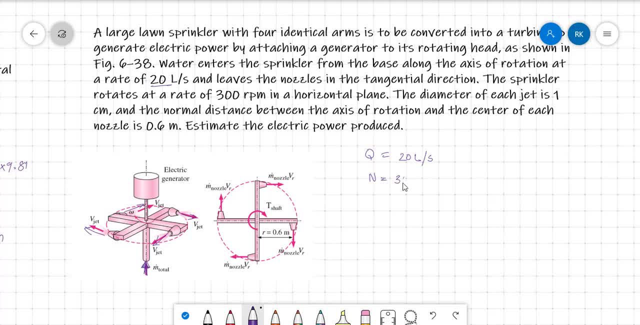 so speed equal to 300 rpm. the diameter of each jet diameter is equal to 1 centimeter, which is equal to 0.01 meter, and the normal distance between the axis of rotation and center of each nozzle is r is equal to 0.6 meter. so what do we need? 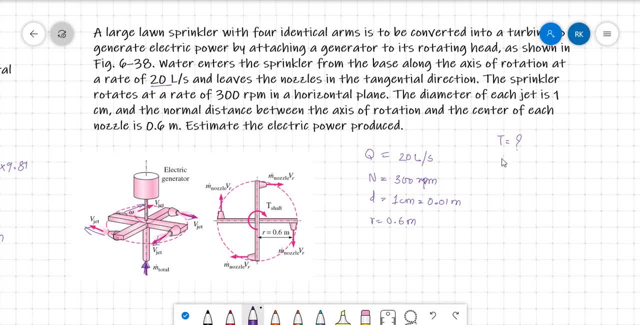 to find. we need to find torque, we need to find Omega, so that power is equal to torque into angular velocity. so angular velocity is equal to Omega, is equal to 2 pi n by 60, so that will be 2 pi into 300. divided by 60, that will be 31.42. 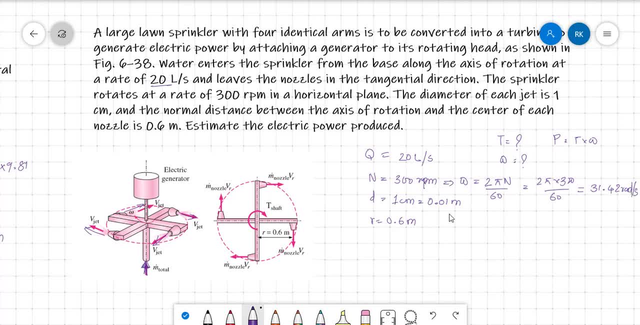 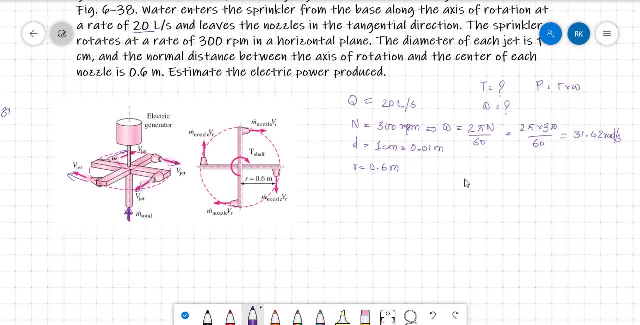 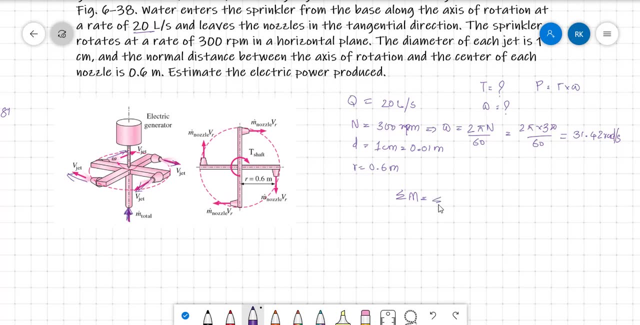 radian per second. so that is 31.42 radian per second. and what else do we need? we need to apply momentum equation, so solid moments is equal to fluid moments. m dot, v are. so there is. I am considering this moment about, about this point. 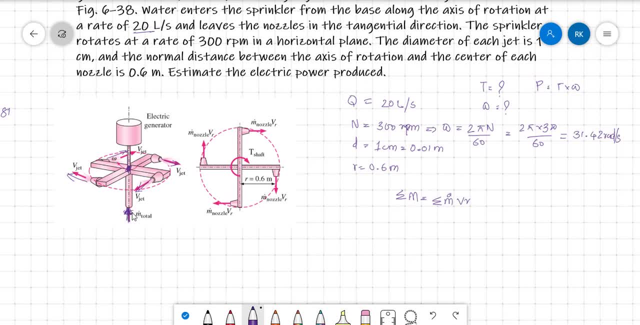 since there is no perpendicular distance of this flow, that is, for zeta during the entrance. so I am the in inward moment. inward momentum is 0, so this is the 높ness value as the outward moment and mass flow rate. mass flow rate is equal. 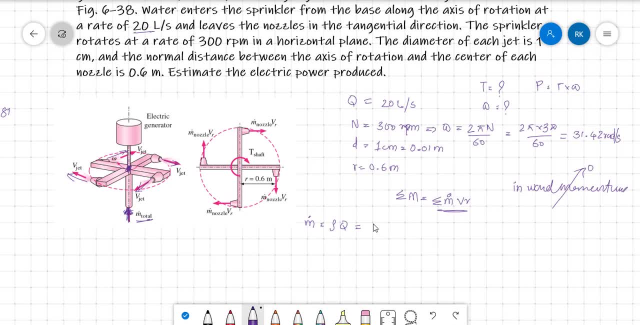 to rho q, where is 1000 kg per meter into 20 liter per second. 20 liter per second, so 1 liter is equal to 1 by 1000 meter cube, so that will be 20 kg per second. so m dot we got. and what is the? 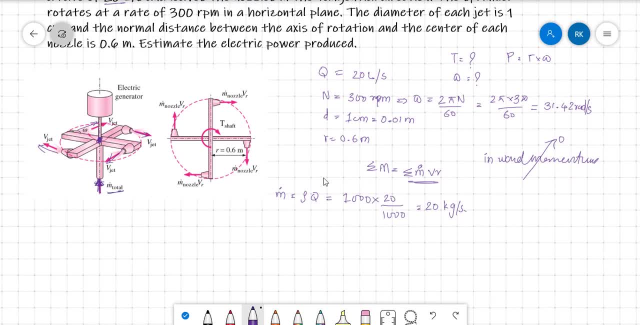 velocity. so velocity will be so tangential velocity. so with what velocity? with respect to nozzle? with respect to nozzle, with what velocity it is coming outside. sorry, that is V jet. jet velocity is equal to. we know that discharge is equal to a into V, so velocity of jet will be discharged by. 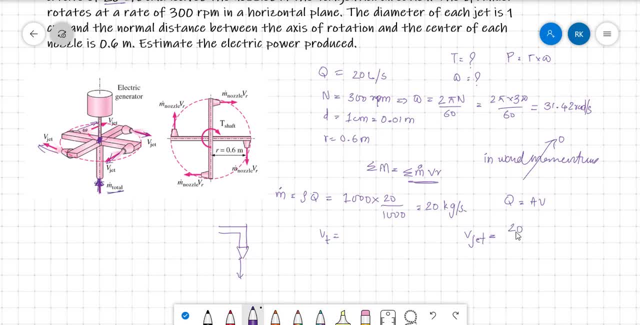 area, so discharges 20 liter per second divided by. so discharge through one, through one nozzle, is: how many nozzles are there? four nozzles are there, so discharge will be distributed. and 20 by 4 will be discharged through one nozzle divided by. 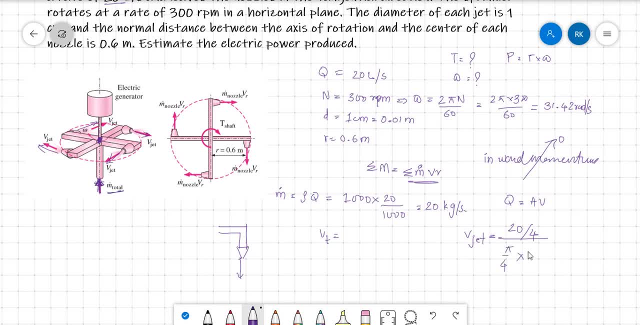 area pi by 4 into d square. d square is zero point zero one square, so this is in liters. so in order to convert into metal cube, that will be divided by thousand. so velocity of jet is sixty three point double six meter per second. and what is a tangential velocity, the velocity of jet? 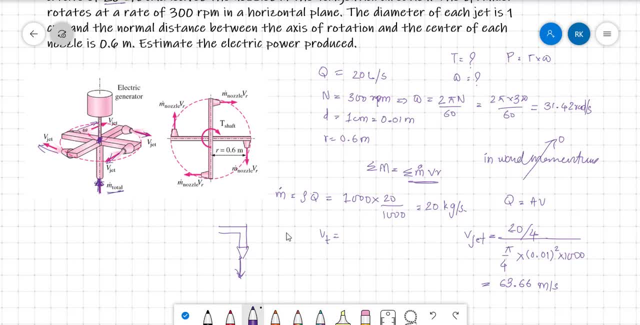 with respect to nozzle is 63 point double-six, and with respect to, if we observe from the ground, that will be absolute velocity. so in order to find the absolute velocity first, we need to find this tangential velocity. so there are four nozzles like this. due to this, there is a opposite. 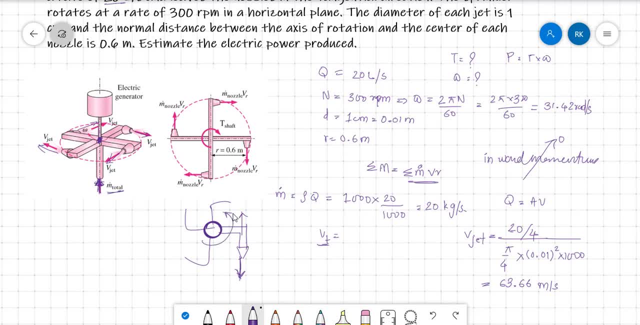 impact that will be created and the rotation is in this way. so, due to that rotation, R, Omega will be the velocity, so tangential velocity is equal to R- Omega. R is 0.6 meter and Omega is 31.42 radians per second, so tangential velocity, tangential velocity of the nozzle will be 18.85. 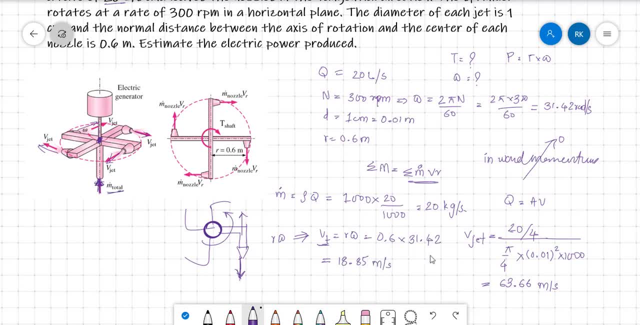 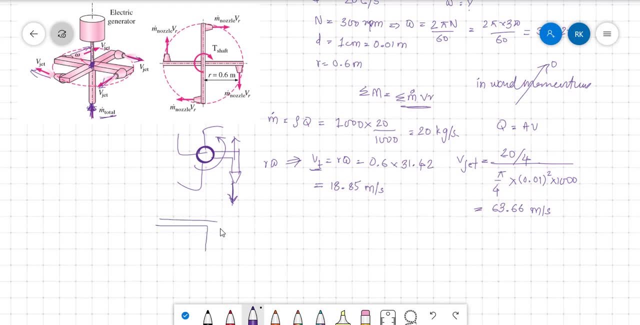 meter per second. so if you observe this velocity, so velocity of the jet is in this direction and tangential velocity of the jet is in this direction and tangential velocity, due to this angular rotation, there is a tangential velocity. in this way, we need to find the absolute velocity, or sometimes it is called as a. 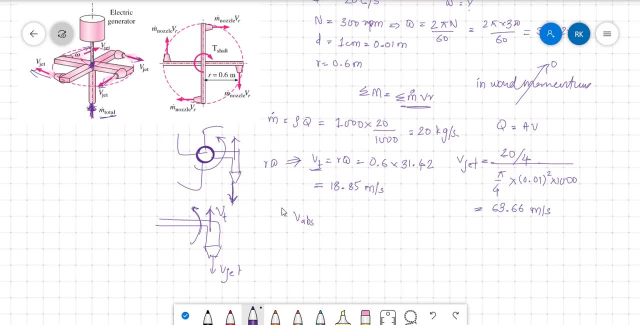 relative velocity with respect to earth. so absolute velocity will be V jet minus V tangential. so V jet is 63.66 meter per second. minus VT that is 18.86 meter per second. so that will be 44.81 meter per second. so the if you observe from earth, it appears like the fluid is coming with. 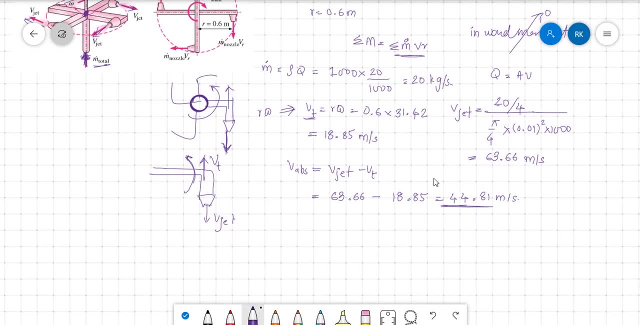 44.81 meter per second. so what do we need? torque? so torque, how do we find torque? Sigma m is equal to Sigma m dot vi H ہ. so what are the solid moments? there is only one solid moment. that will be the resistance due to the generator. so that will be torque. the needed torque will be. 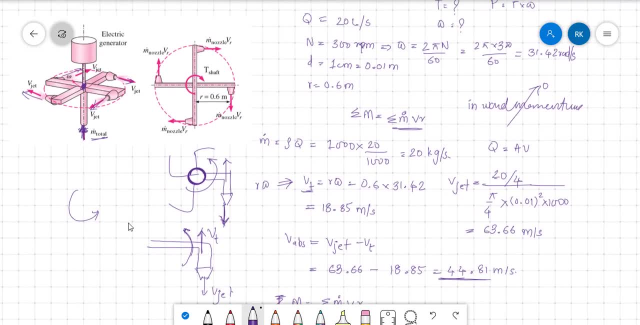 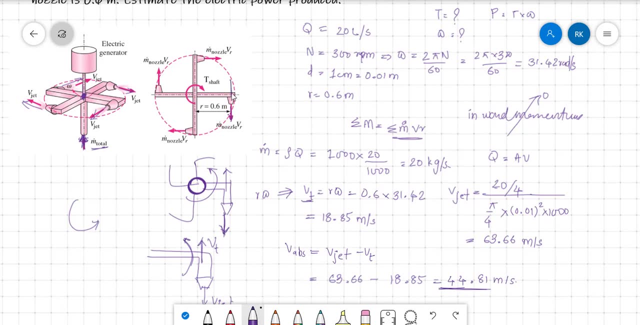 in which direction? so, as I said, if the velocity is in this way, there is a opposite impact that will be created on this body and due to this opposite impact, there should be a resisting torque, so that will be in clockwise direction. if this is anti-clockwise one, so there is clockwise one, so torque is clockwise, considering clockwise as. 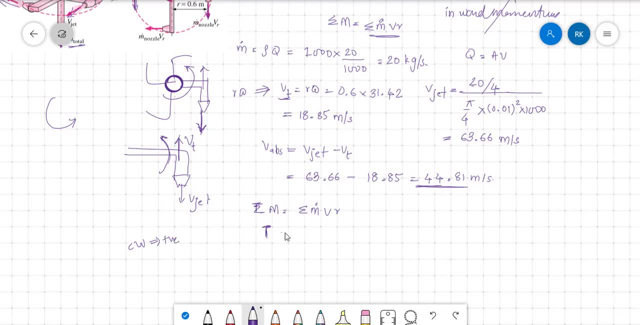 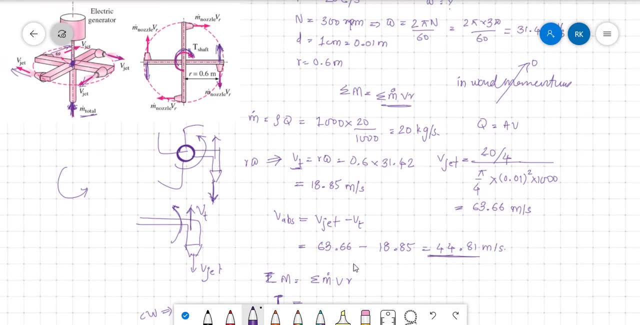 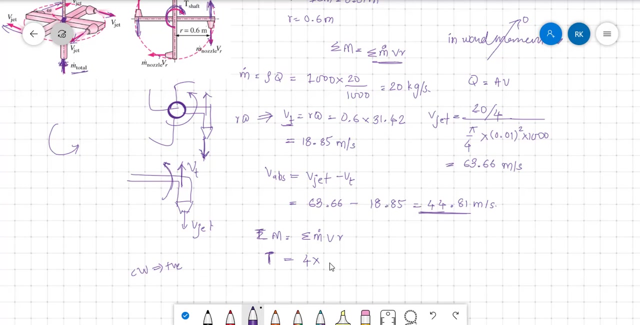 positive. so T is equal to. so how many exits are there? one, two, three, four, four. four exits are there, so 4 exits means 4 into, since all the mass flow rates are equal and the radial distances are also equal. so I am multiplying it with 4 M dot we. 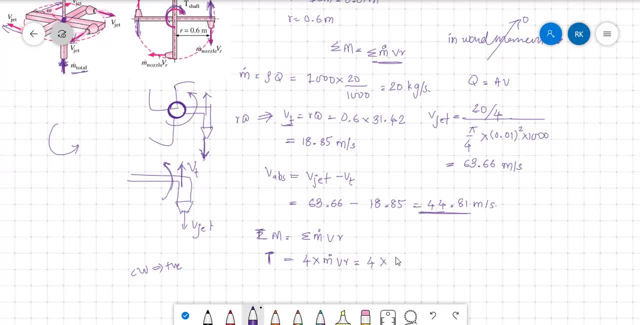 are. so 4 into M dot. what is mass flow rate? this is 20 kg per second. 20 kg per second, but it is a total mass flow rate and through single nozzle that will be divided by 4 into velocity. with what velocity? absolute velocity is forty four. 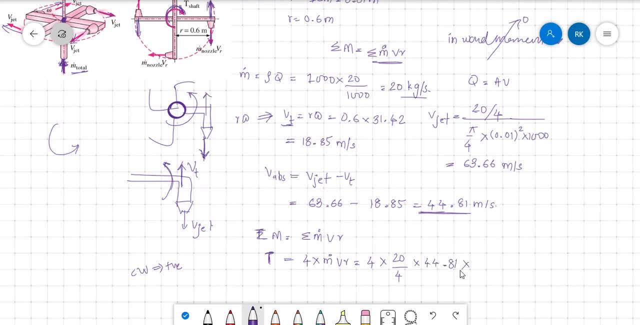 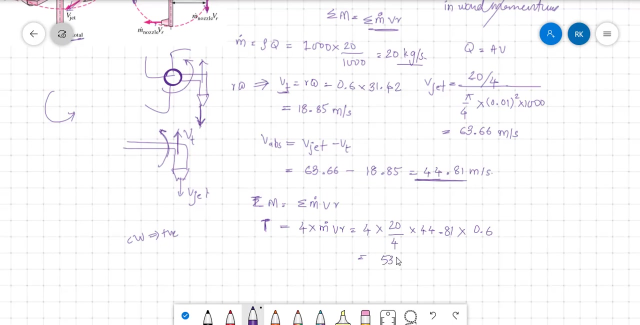 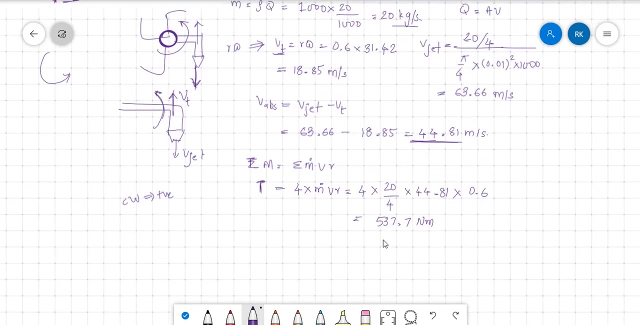 point eight. one meter per second into the radius is 0.6. so solving this torque we will get 537.7 Newton meter. so talk is this much. and what is power? power is equal to T into Omega, torque, 537.7 into Omega. what is angular velocity? angular velocity, we. 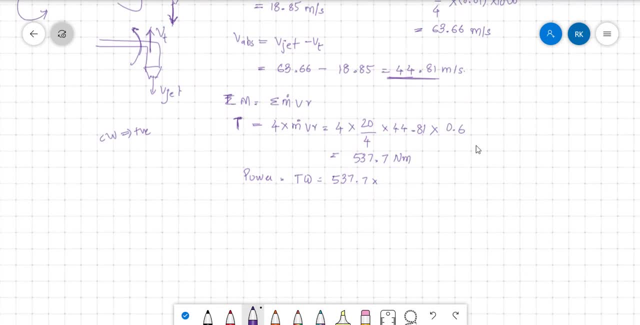 got it as 30.7, 30.7, 30.7, 30.7, 1.42 radians per second. so divided by thousand gives us power in kilowatts. so sixteen point nine kilowatt is the answer. so this is all we need to. 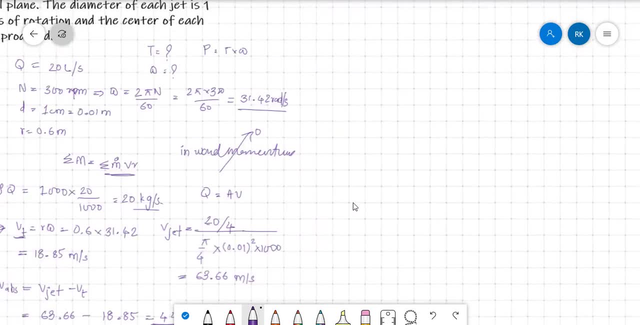 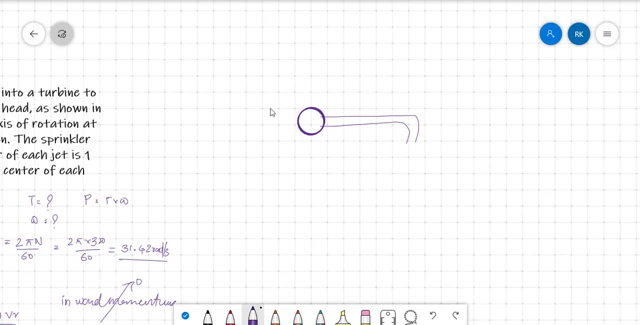 solve lawn sprinkler problems. and also let me say one thing: so if the lawn sprinkler is in this way and the velocity of jet coming like this, so due to this there is an opposite impact that will be created and due to that rotation will be in this way. so due to this there is V tangential, so V absolute is equal.